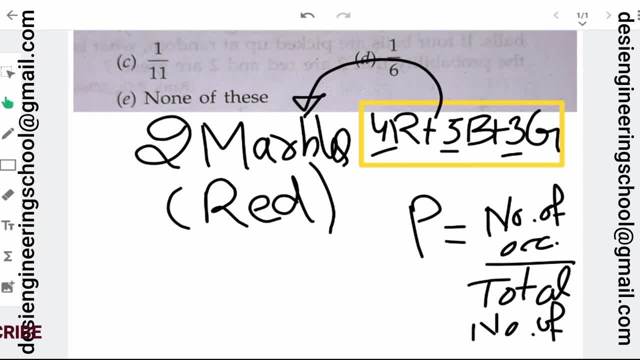 From these 12 marbles. any one marble can be removed. Any one of our barmers can be out. So what is the total number of events? We have 12 for the first time, If we talk about the first marble. If we talk about the first marble, 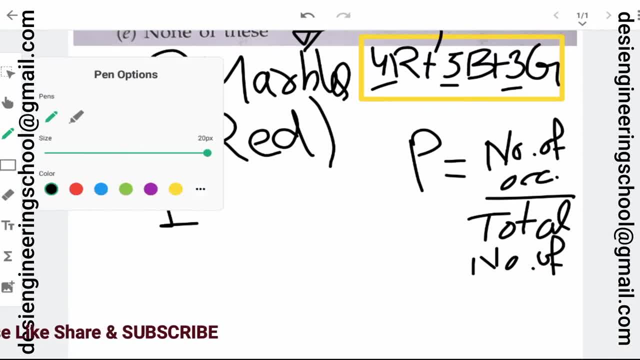 Suppose we are drawing the first marble. So If we take out the first marble, then the total number of events will be 12, Because any one can be removed from here Now it will be red. what is its probability? So this 4, if any one of these 4. 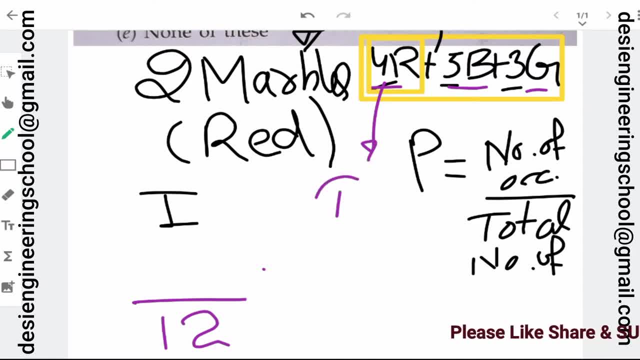 is removed. okay, If any one of these 4 is removed, then that means our marble will be red. That is our occurrence, That is our expectation, That is your probability. So from here we have 4 red marbles Now The second time it withdraws. When it withdraws the second time, randomly. 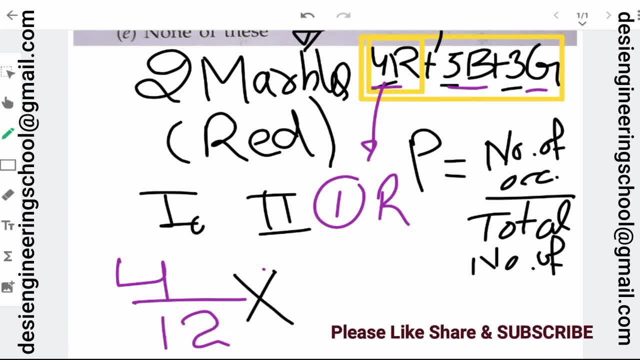 It is doing it randomly. That is why it will multiply, Because we are doing it continuously. We are doing it first and then second time. Now what is in the second time? So see what is in the second time. After 4 red marbles, how much is it now? 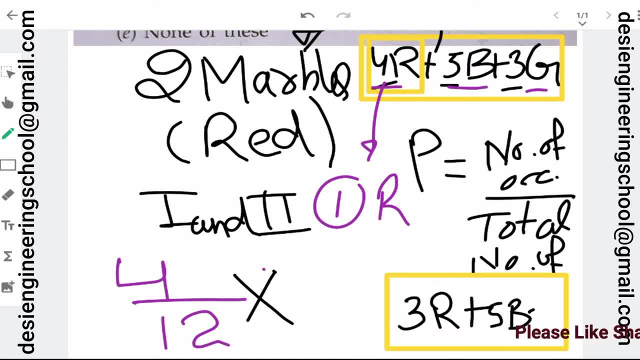 3 red, 1 is already removed. Plus 5 blue. plus 3 green: 1 is already removed. That is why we have done here, That is why we have written 3 here, That is why we have written 3 here, Because already 1 red has been removed. 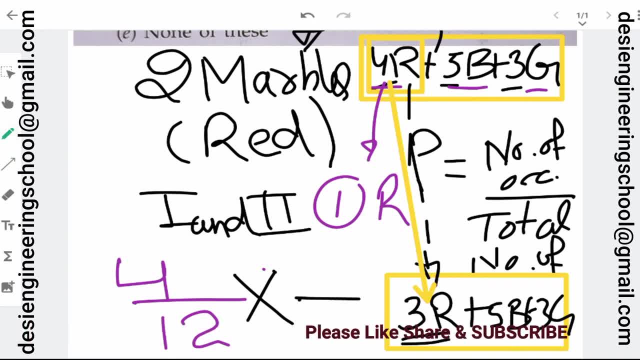 So 3 red is done. Now what is our occurrence? Total number of events: 3 plus 5 plus 3 Will be 11. And then what is the probability That, from here, If any one of these 3, If any one of these 3, 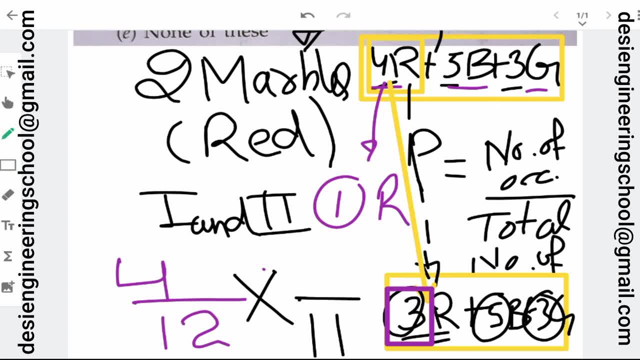 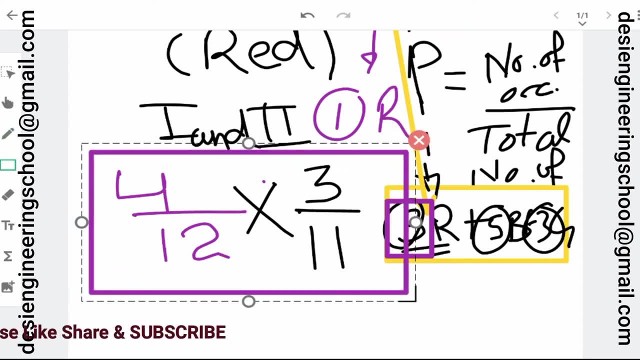 If any one of these 3 marbles, If any one of these 3 marbles, If any one of these 3 marbles, Then that will be your occurrence. So here the probability will be 3. So why did it multiply? Why did it take 4 here? 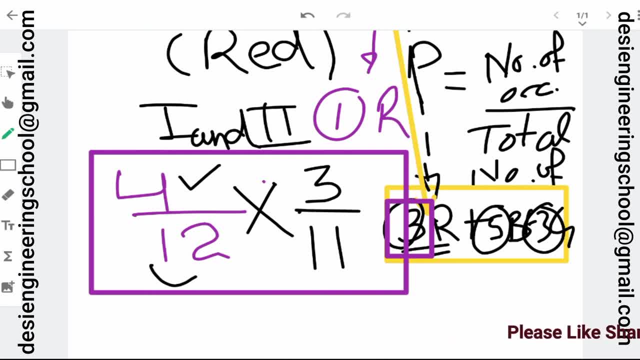 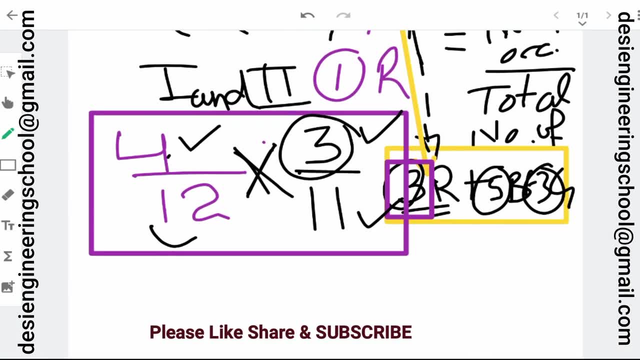 Because any one of the 4 reds- That is our probability And 12 is the total number of events. What is in the second time? If 1 is removed, then only 3 reds are left, So 3 and 11 out of the total number of events.